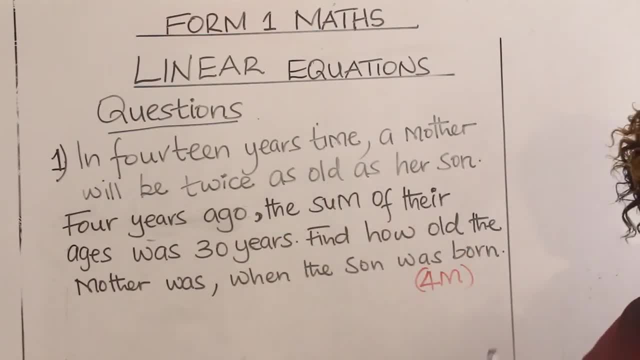 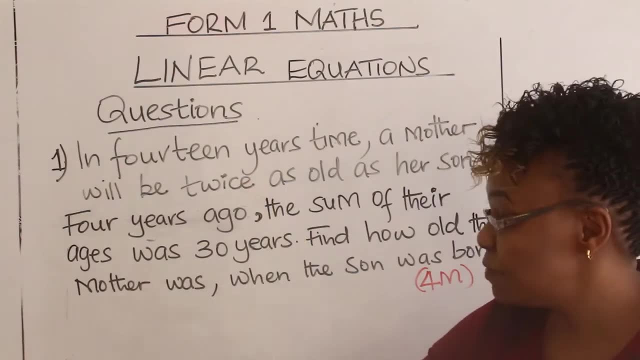 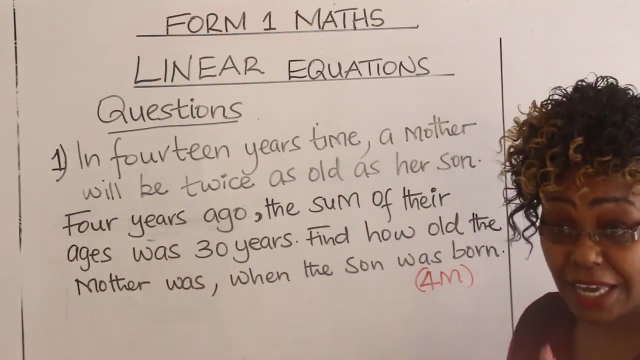 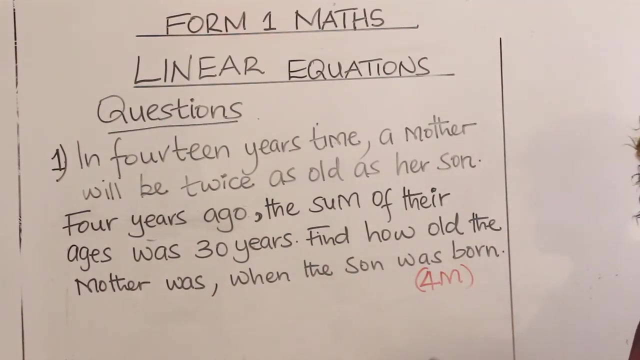 will be twice as old as her son. In 14 years time, a mother will be twice as old as her son. That one is talking about the future. Four years ago. we are now talking about the past. the sum of their ages was 30 years. Find how old the mother was when the son was born. How old the mother was. 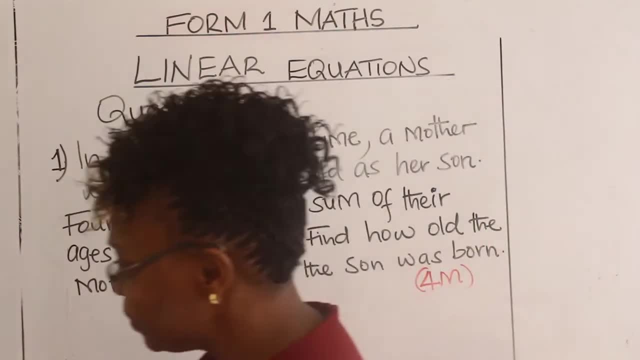 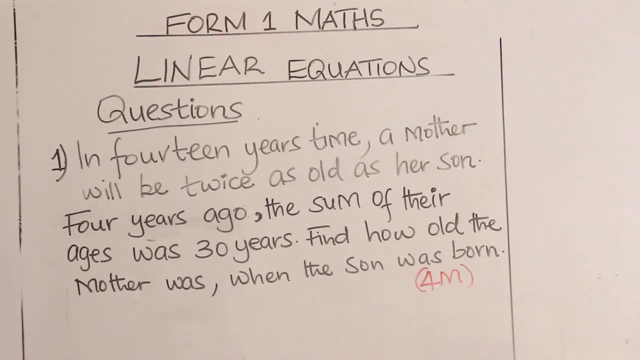 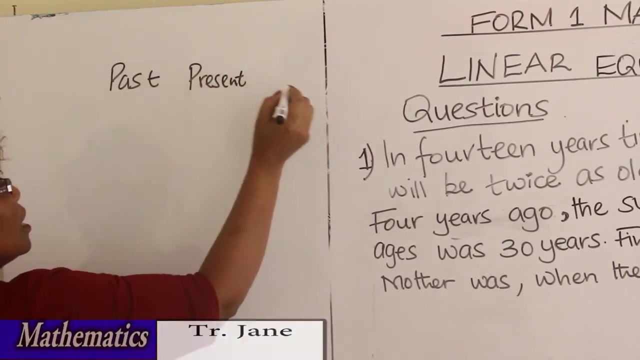 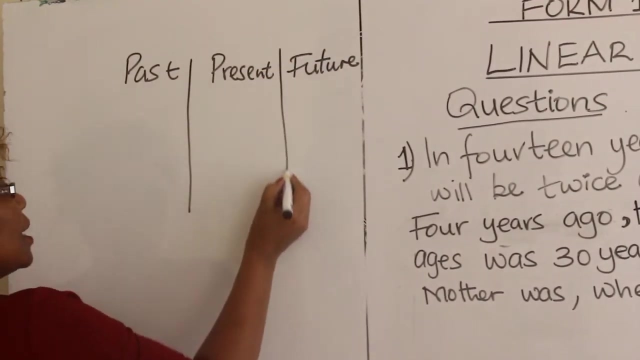 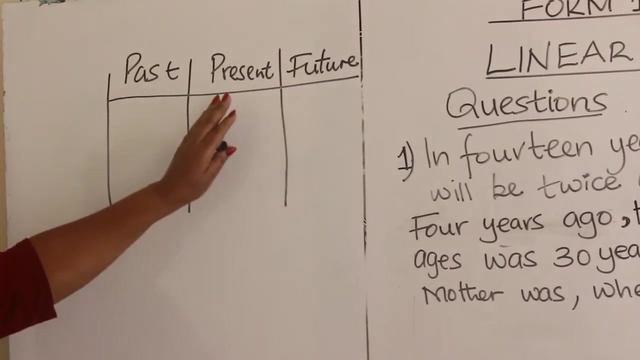 when the son was born. How do you go about this? What you do is that you draw three columns. You draw three columns, Here you have the present and here you have the future. You have the future Like that, Like that, Lana. So you go to your question. You have the present. 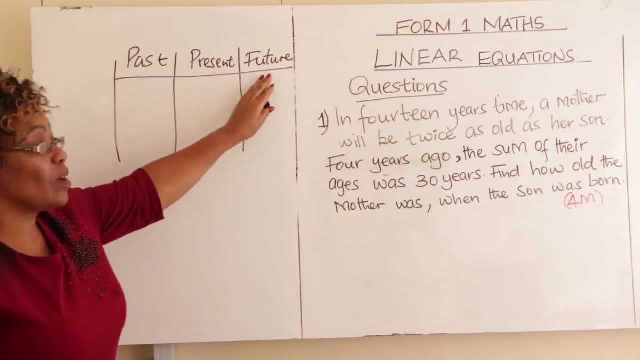 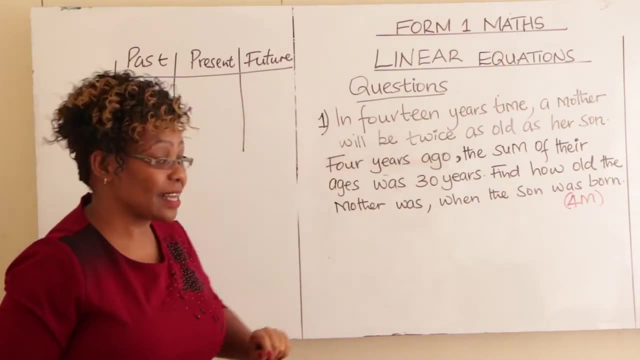 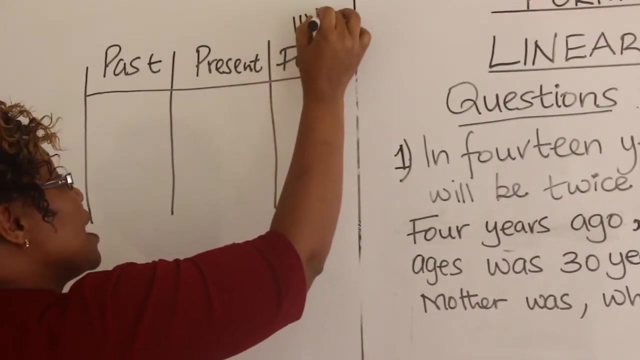 today. past is a go, and then you have the future. So in 14 years time, Lana, a mother, will be twice as old as her son. You come to this because that one is talking about the future. You come and write here 14 years time. 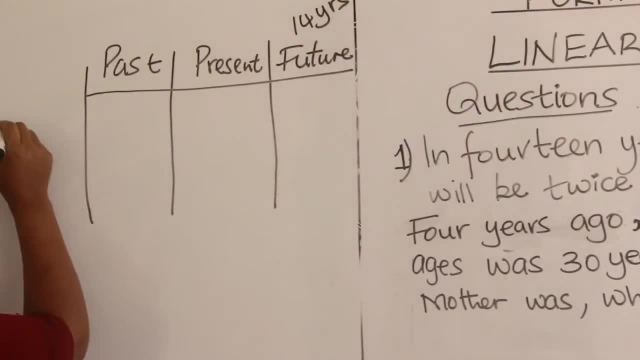 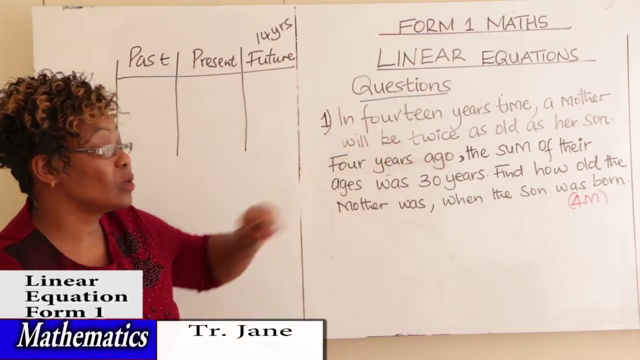 In 14 years' time, the mother- you come and write the mother here, and here you write the son. So in 14 years' time you go to that column of the future: the mother- a mother- will be twice as old as her son. 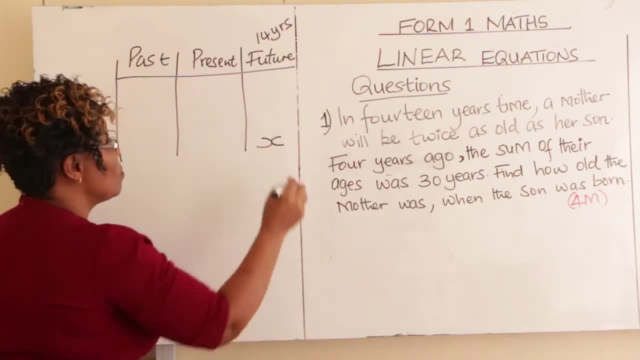 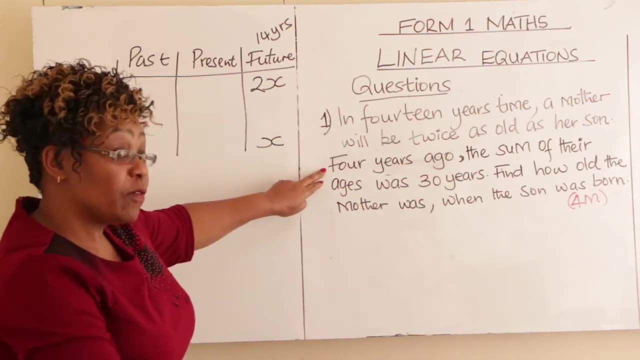 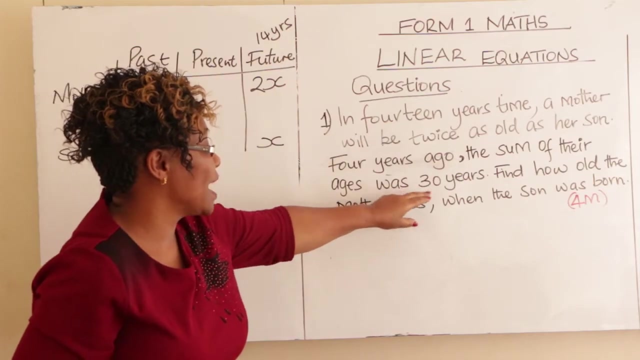 So if the son will be X years, the mother will be 2X. The mother will be 2X. Then you come here. 4 years ago- this is now to do with the past 4 years ago- the sum of their ages was 30.. 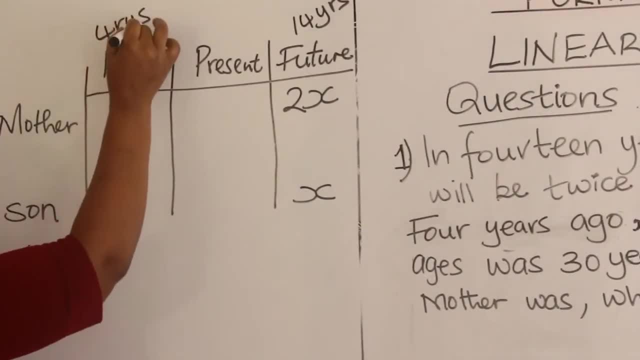 4 years ago here 4 years ago, sorry, 4 years ago. the sum of their ages will be 30, it will add up to 30. So how do you go about that? Find how old, how old the mother was when the son was born, when the son was born? 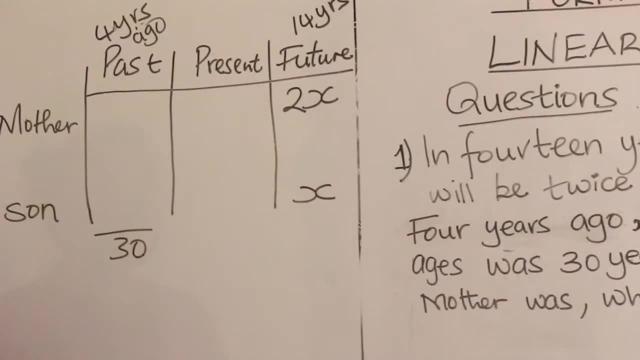 So how do you go about this? You come to the future. You say: if in future the son will be X years, what about today? What about the present? It will be X minus 14,, X minus 14.. You subtract because you're talking about the future here. 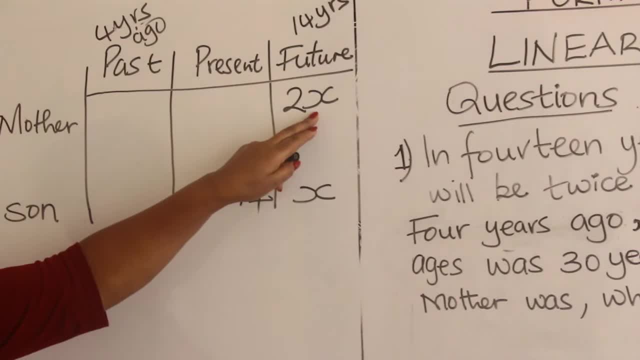 So in the future the mother will be 2X years. In 14 years' time the mother will be: the mother will be 2X. So to get the present here, Lana, you subtract 14 also, So you'll talk of 2X minus 14.. 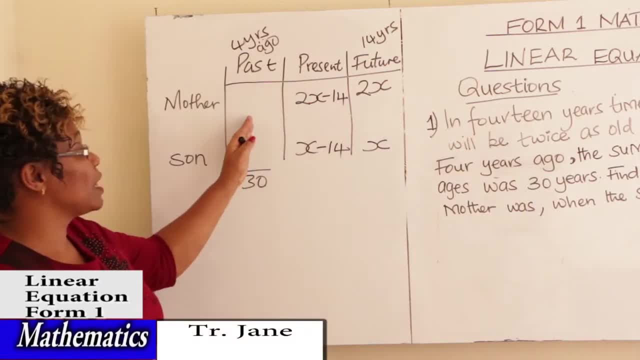 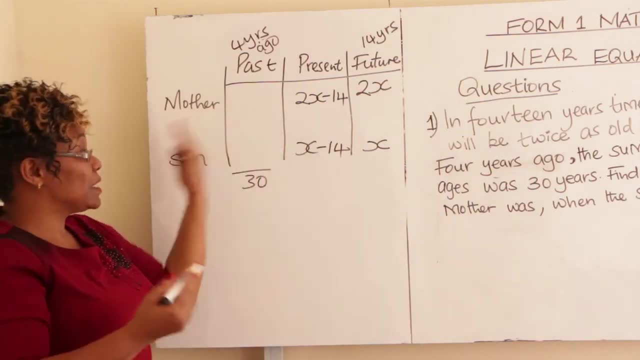 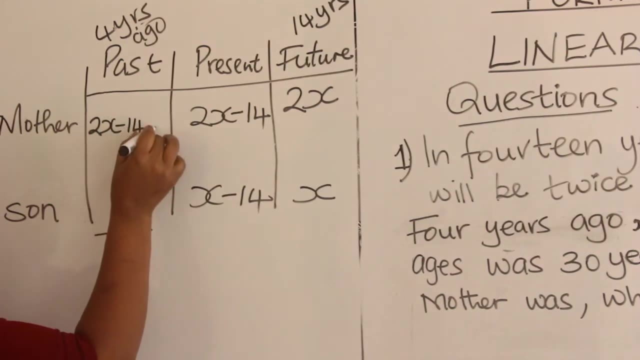 So these are their ages today. Then you now go to the past here. If today the mother is this old, what about 4 years ago? You subtract again, you subtract 4 years And therefore the mother will be 2X minus 14, minus the 4 years. 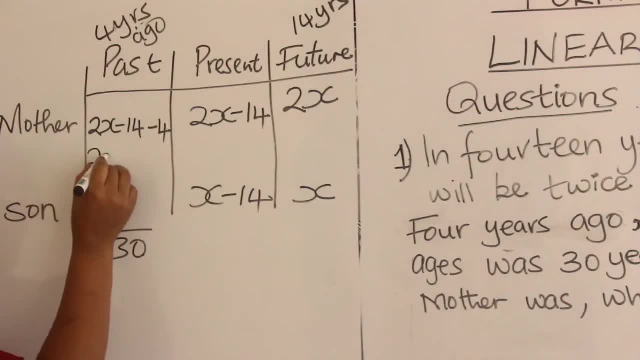 And therefore this gives us what This will give us: 2X minus 14 minus 4. It will give you minus 18.. So you come in here to be a minus 18.. We go to the son Today. the son is X minus 14 years. 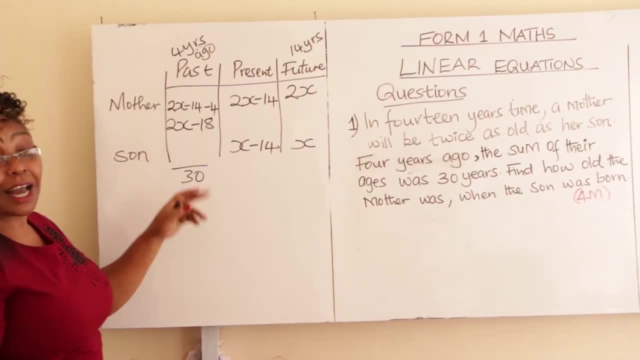 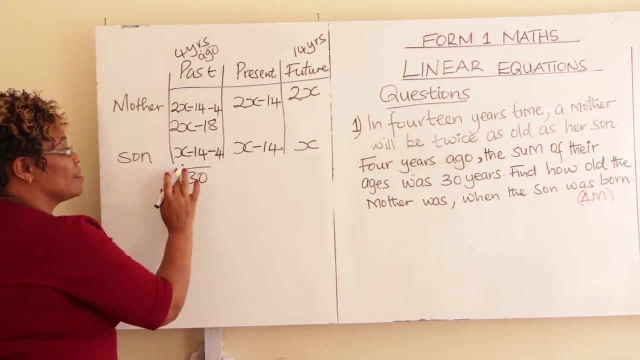 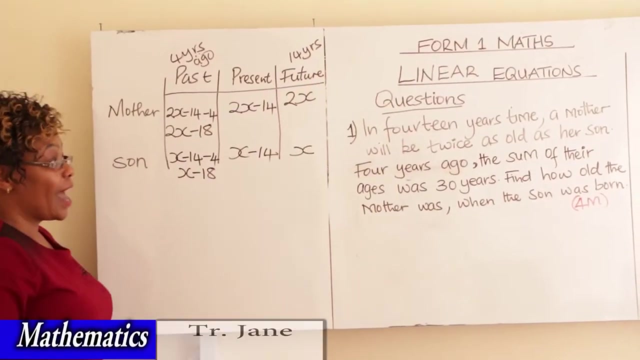 So 4 years ago, the son was: how old? Again, you subtract 4.. So it will be X minus 14 minus 4 years, And this would give you what this would give you again: x minus 18, and therefore we are being told. 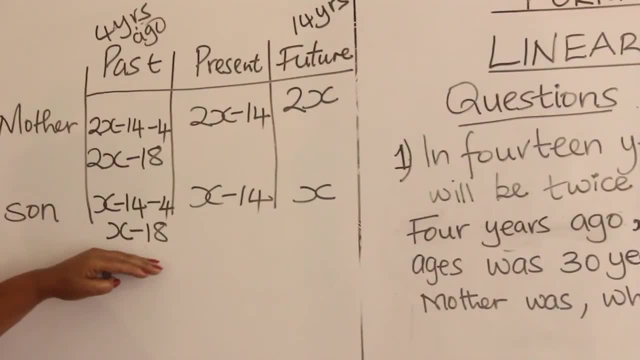 that this age plus this age 4 years ago would add up to 30 years. the sum of their ages was 30 years. so this plus this would give you 30 years. so you come and add the 2 lambda, you add the 2 divide that. 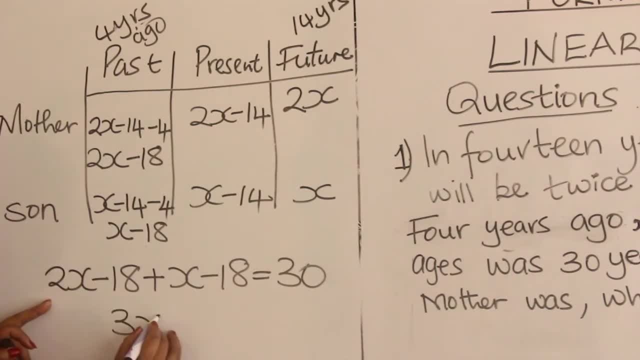 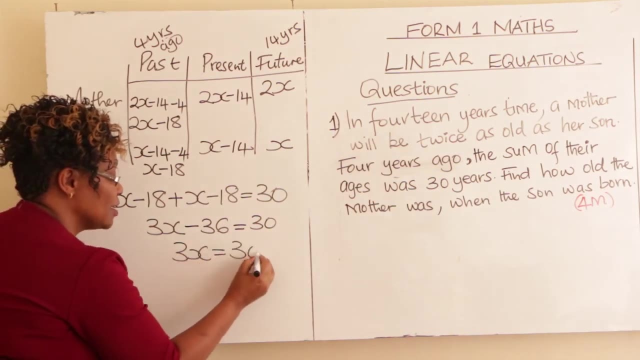 you bring the like terms together there: minus 18 minus 18 is what. minus 36 minus 36 gives you 30, and therefore this is 3x is equal to 30 plus 36, and therefore this is 3x is equal to 66. 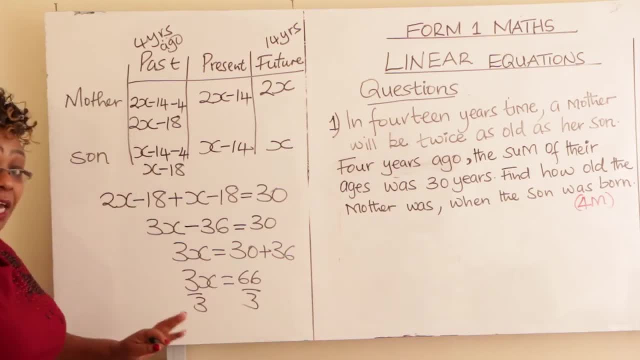 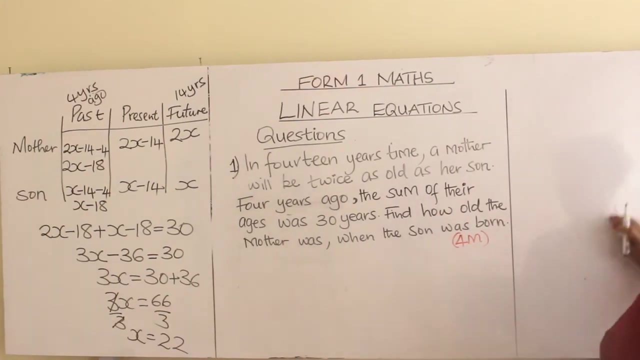 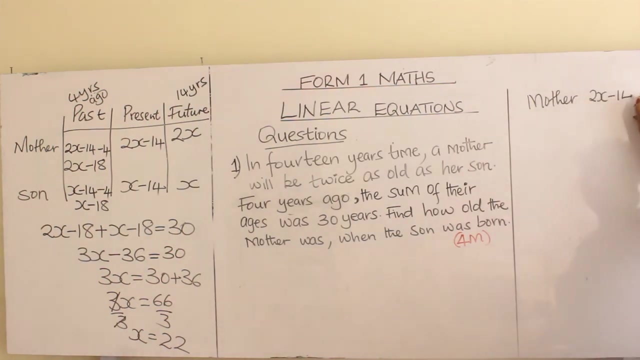 divide by 3. divide by 3 to get your x and therefore x. what is your x? your x is 22. your x is 22. so you go to their present ages. how old are they today? you look at the mother. so the mother today is 2x minus 14.